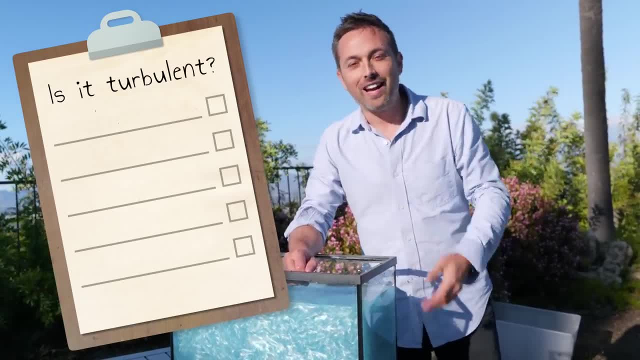 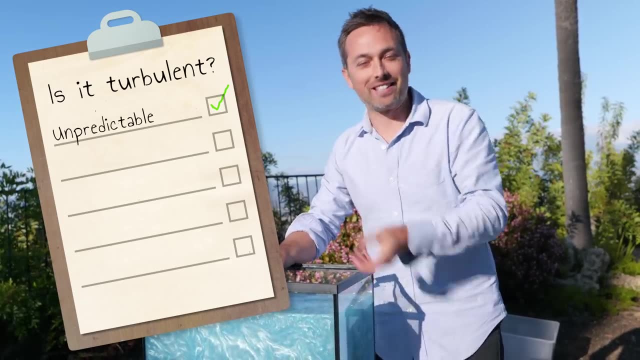 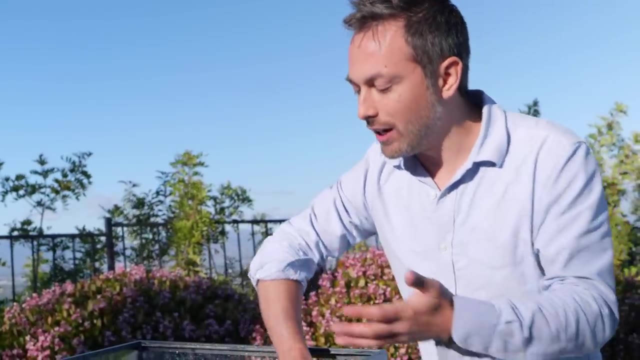 characteristics of turbulent flow, so that you know it when you see it. And the first characteristic of turbulent flow is that it is unpredictable. That's right, Turbulent flow is messy, It's unpredictable. It is literally, definitionally chaotic, meaning it is sensitively dependent on initial conditions. 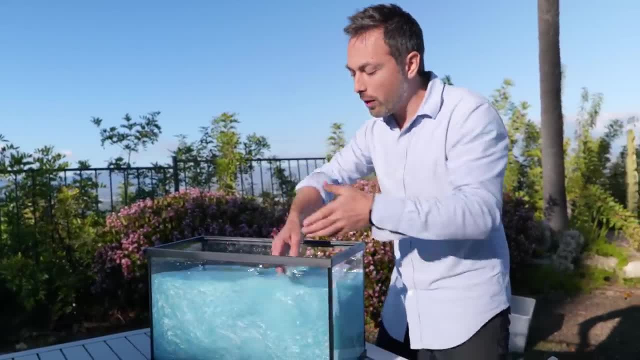 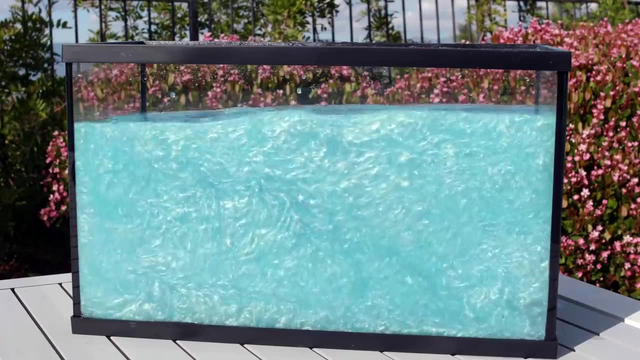 So if you were to change something somewhere in the fluid, well, it would completely change the final state, And that means you can't make predictions with turbulent flow. All you can do is speak about it statistically. I mean, there are the Navier-Stokes equations which are meant to govern. 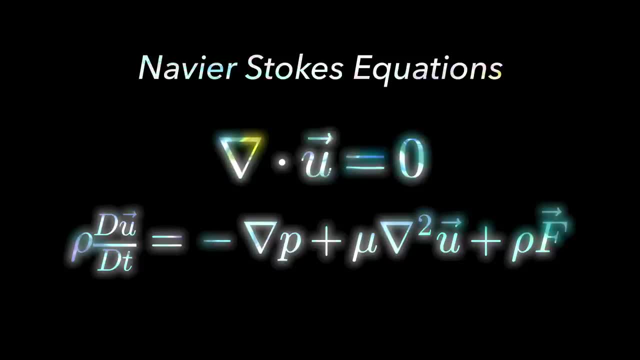 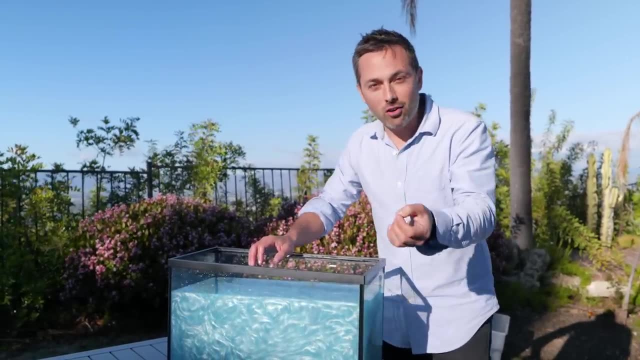 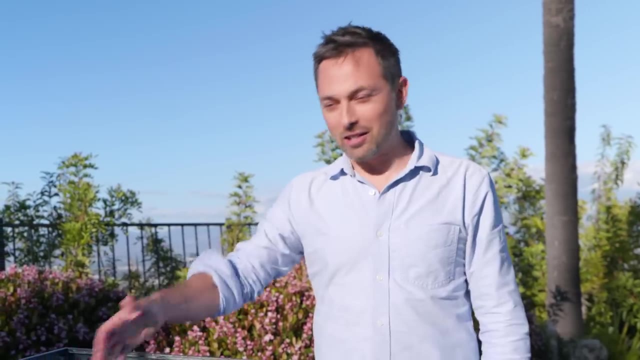 all fluid flow, including turbulence, but they are notoriously difficult to solve. In fact, there is a million dollar prize for anyone who can even make progress towards getting insight into these equations. that would explain turbulence. So yeah, I get it: Turbulence is a mess. Laminar flow is easy to love: It's like the bell of the ball. 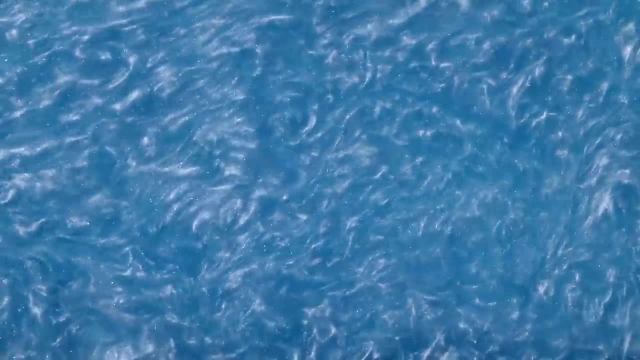 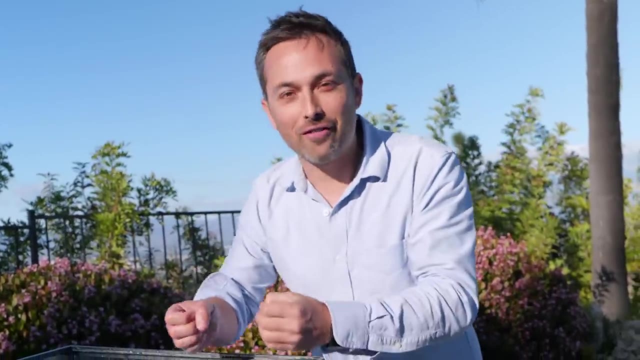 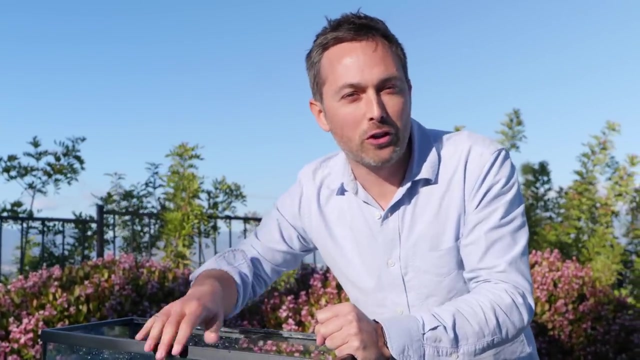 whereas turbulent flow is kind of an ugly duckling, But in this video I want to transform that ugly duckling into a beautiful swan. I want you to see that if you make the effort, the love you can have for turbulent flow is so much deeper and richer than that superficial fling you have with laminar. 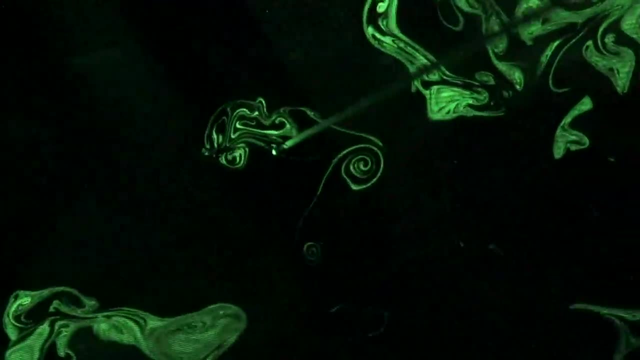 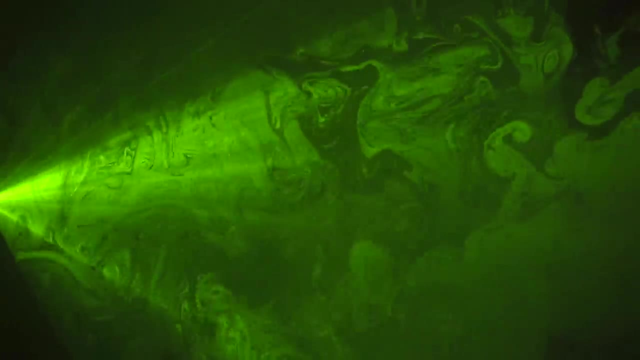 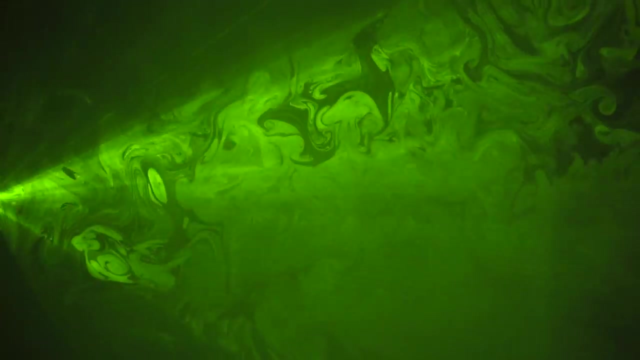 flow. You are looking at the motion of air in a room which is generally turbulent. The physics girl and friends imaged a cross-section of air using a fog machine and a laser sheet. One of the defining characteristics of turbulent flow is that it consists of many interacting swirls of fluid. 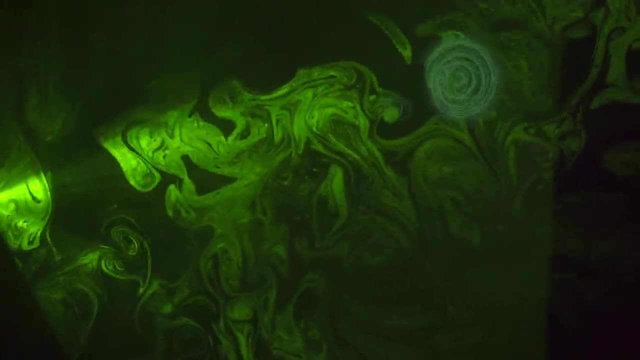 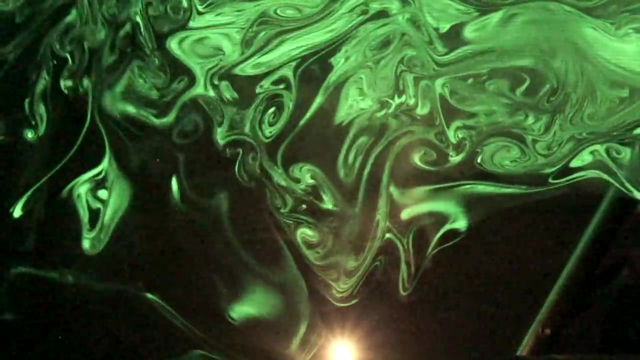 also called eddies or vortices. These eddies span a huge range of sizes- In the case of air in a room, from the micrometer scale all the way up to the speed of light. the speed of light is about. 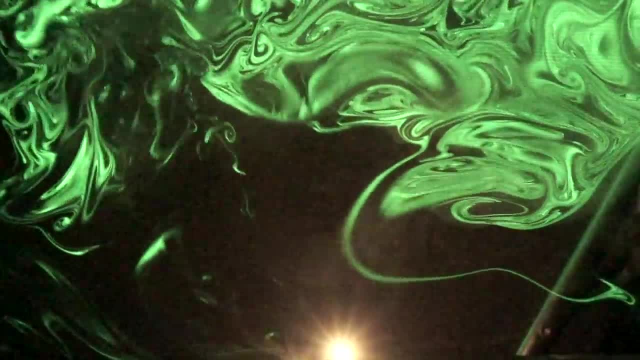 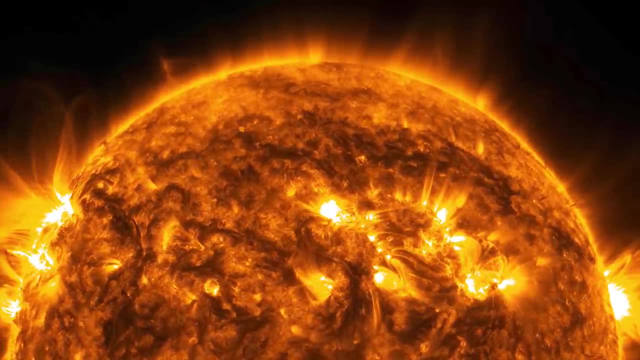 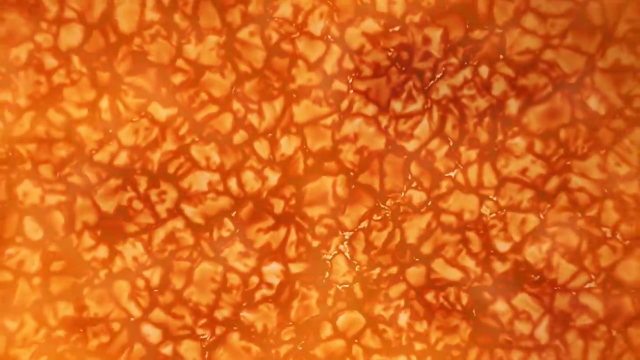 meters in diameter. Can you think of another physical phenomenon that exhibits structures over such a range of sizes? But turbulence can be much larger. The surface of the sun is turbulent as hot plasma rises to the surface in huge convection currents. The cell-like structures 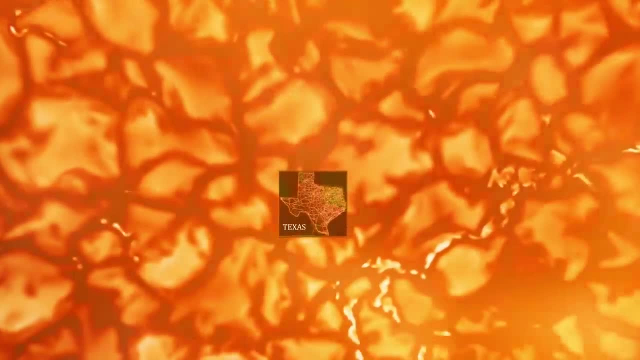 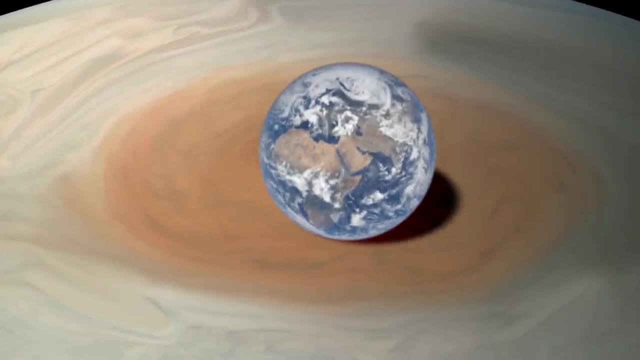 here are roughly the size of Texas. Larger still are the turbulent swirls on Jupiter. The great red spot is a vortex bigger than the earth. The rest of the earth is a vortex bigger than the earth. The rest of the earth is a vortex bigger. 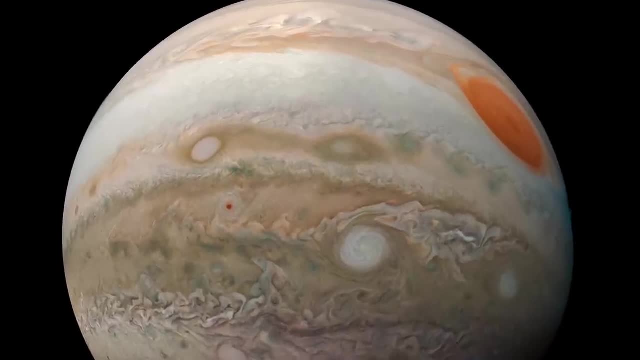 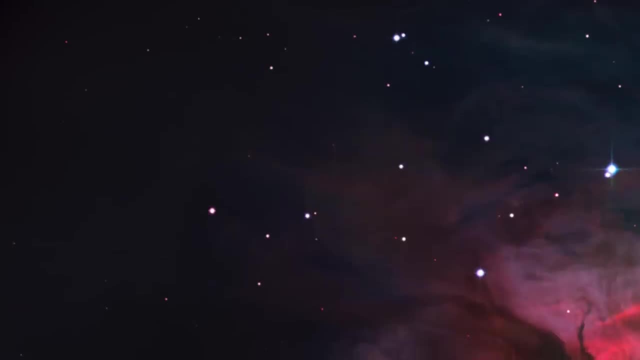 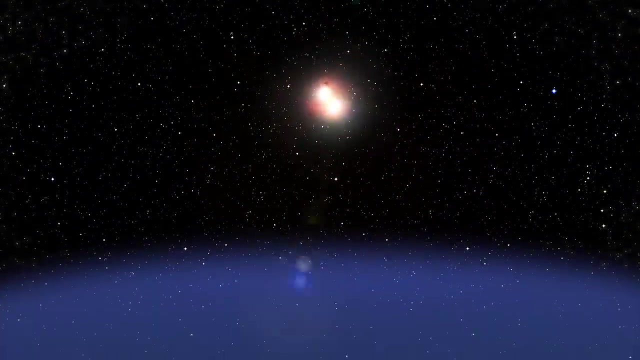 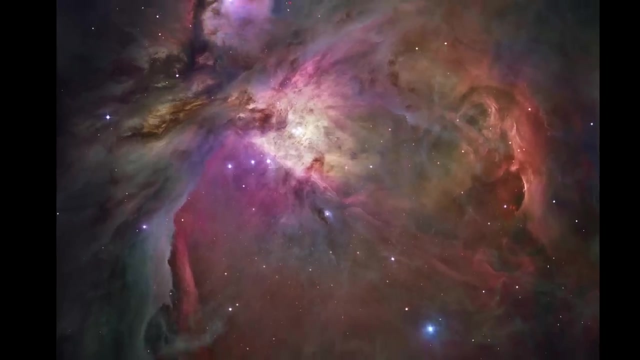 orbiting spacecraft. Even the dust between the stars is in turbulent motion. It makes radio sources twinkle. the same way, the turbulence in our atmosphere makes stars twinkle. A stunning example of this turbulent dust is the Orion Nebula, 24 light years across. Turbulence is cosmic. In contrast, 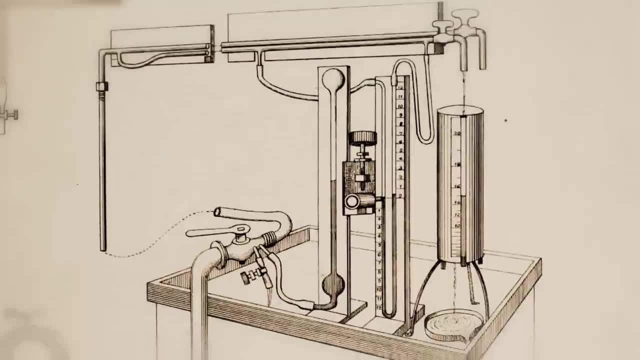 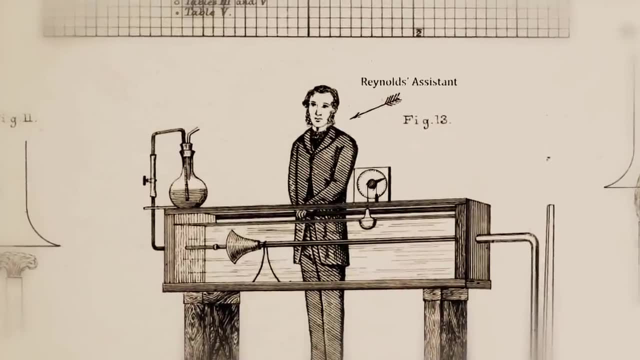 laminar flow has to be small. This was shown experimentally in 1883.. Osborn Reynolds passed water through a glass pipe at different flow rates and to visualize the flow he introduced a stream of dye in the middle of the pipe. He found at low. 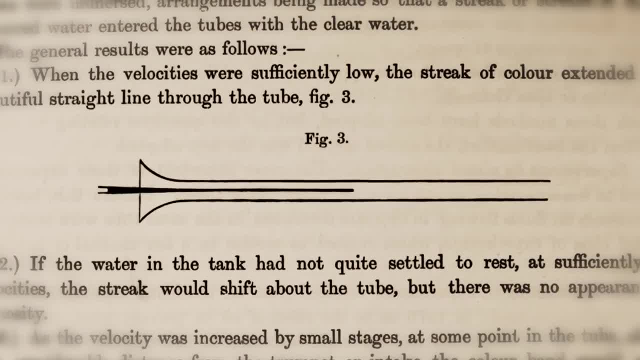 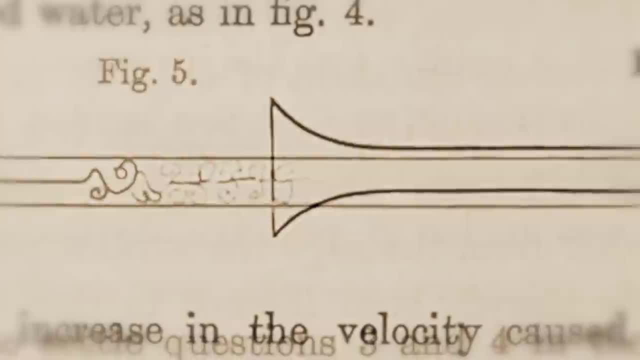 flow rates. the dye remained in a steady stream, laminar flow. But as the flow rate increased, the dye began to oscillate back and forth and beyond a certain critical point, the dye became completely diffused to the surface of the water. The dye became completely diffused to the surface of the water. 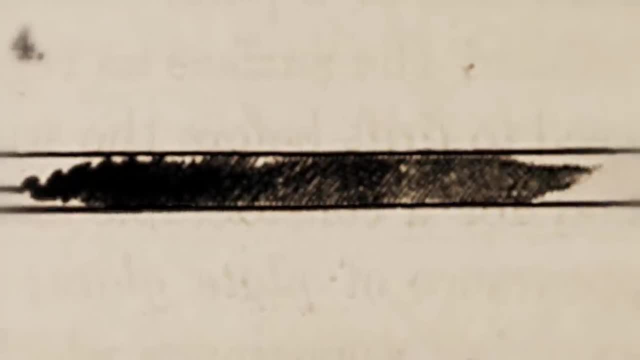 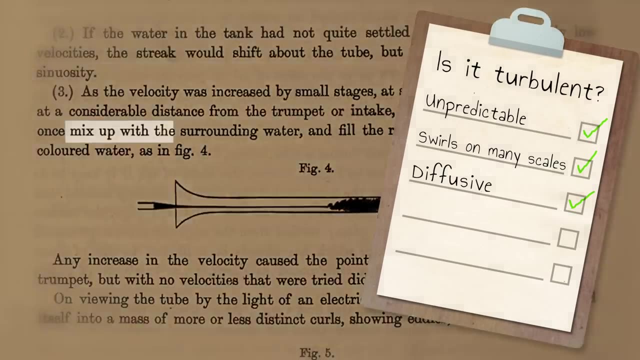 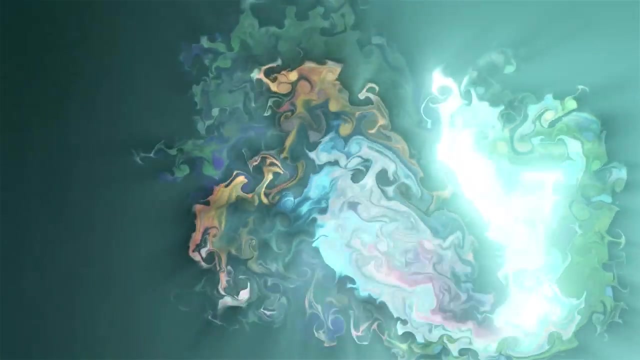 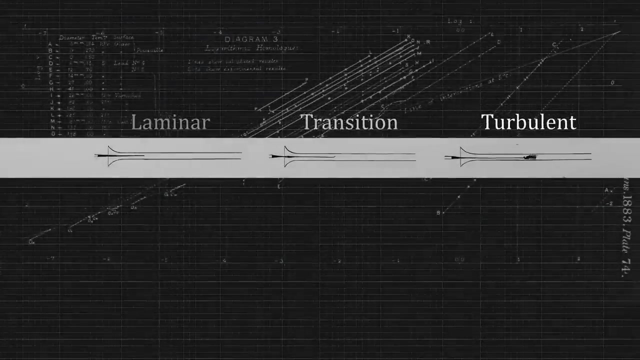 throughout the pipe. this was turbulent flow. reynolds had observed another essential characteristic of turbulence: it is diffusive, meaning it mixes things together. turbulent flows cause things to spread out, not only die, but also heat or momentum. they all become distributed throughout the fluid. reynolds found the transition to turbulence was not only dependent on the flow rate. 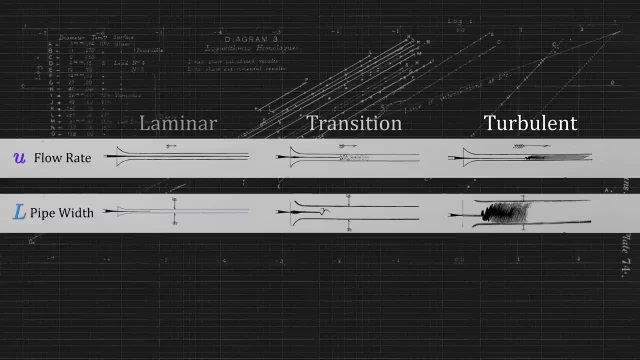 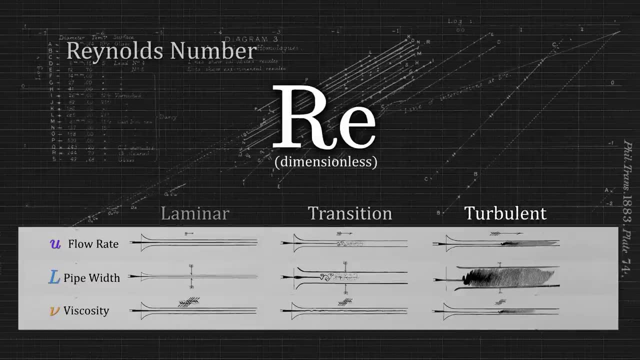 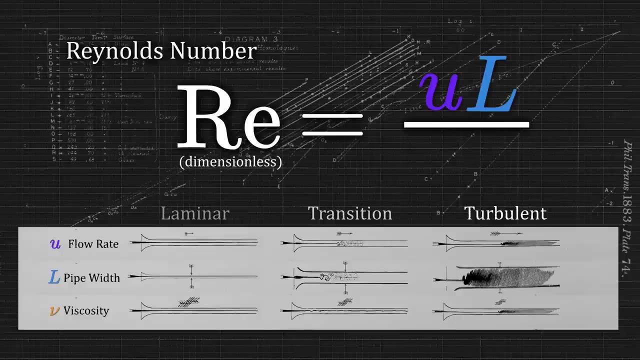 turbulence occurred more readily in wider pipes, but less readily with more viscous fluids, things like honey. he calculated a dimensionless quantity, now called the reynolds number, equal to the velocity of the fluid times, the characteristic length, say the diameter of the pipe divided by the kinematic viscosity of the fluid. 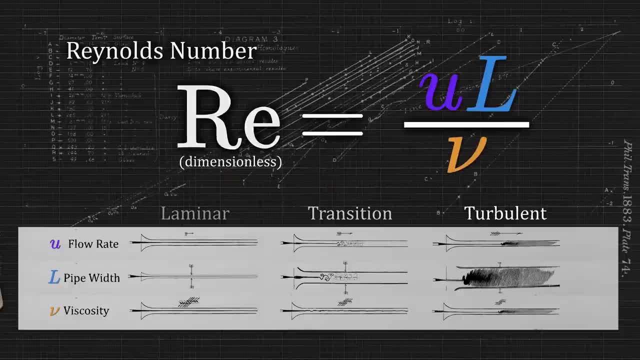 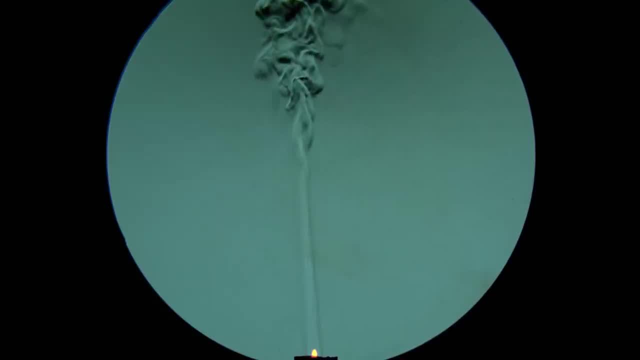 which you can think of as a measure of its internal friction. high reynolds numbers result in turbulent flow. have a look at the smoke rising from a candle flame. at first it's laminar, but the hot gases accelerate as they rise and once the reynolds number gets too big, the smoke transitions. 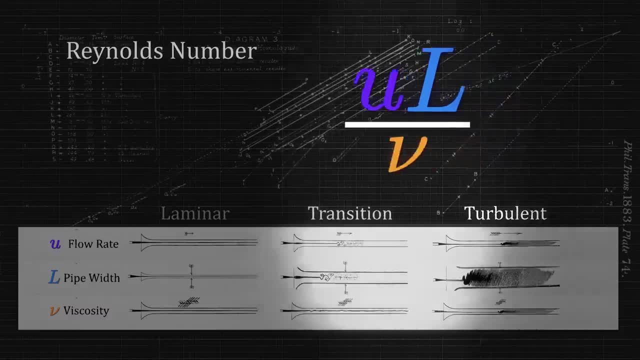 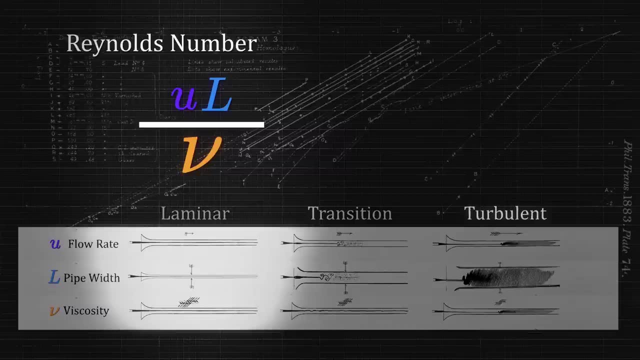 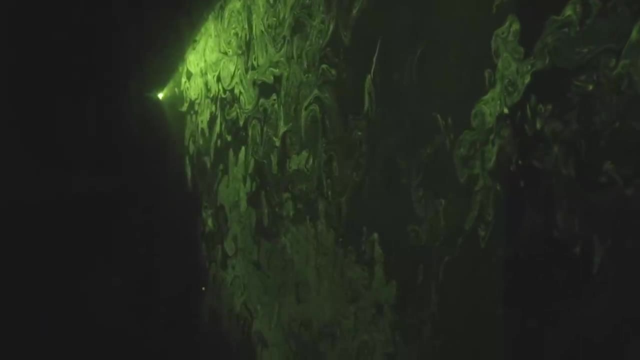 to turbulence. so laminar flow only occurs at low reynolds numbers, which means it is limited to low speeds, small sizes or viscous fluids. this is why in our everyday lives, most fluid flow is turbulent. turbulent flow is the rule, laminar flow is the exception. 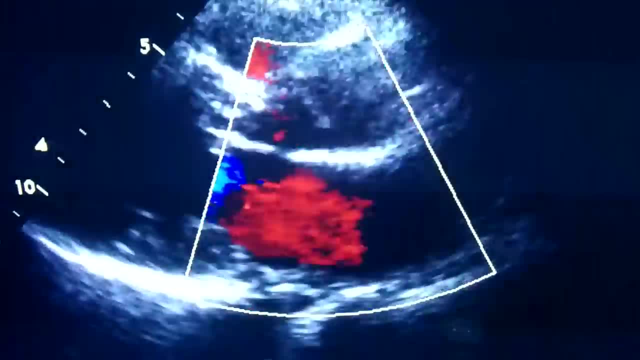 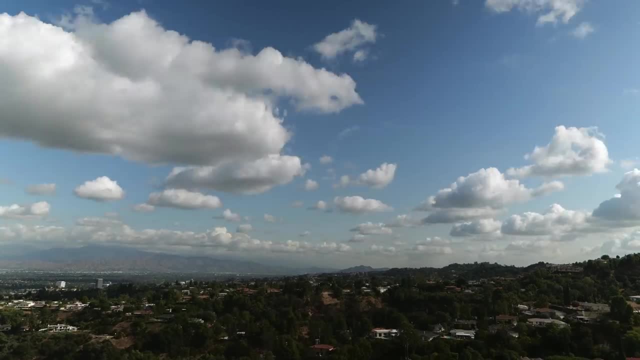 the air flowing in and out of your lungs is turbulent. the blood pumping through your aorta is turbulent. the atmosphere near the surface of the earth is turbulent, as is the airflow in and around cumulus and cumulonimbus clouds. in fact, modeling shows that turbulent flow plays an 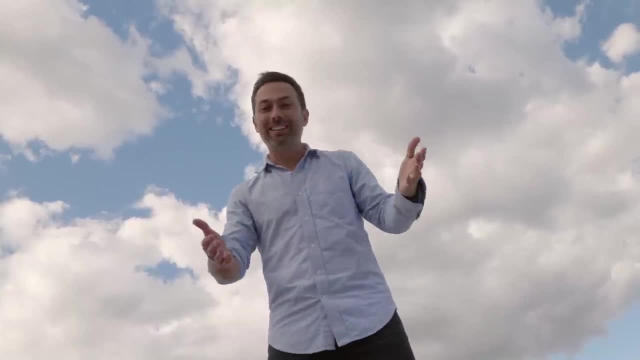 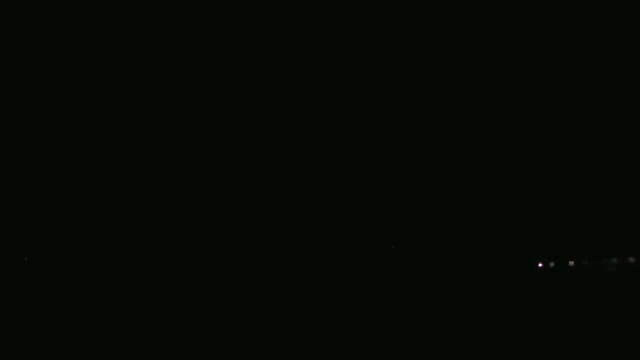 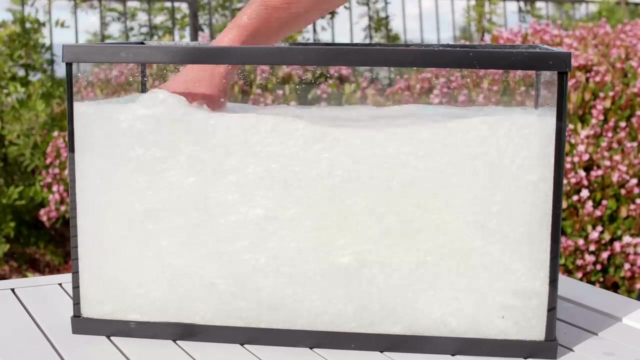 essential role in the formation of raindrops, so turbulence literally makes it rain. i'm going to create turbulence in this rheoscopic fluid. rheoscopic just means that it shows the currents, and it does that by having these tiny particles suspended in the water. but what you notice if you? 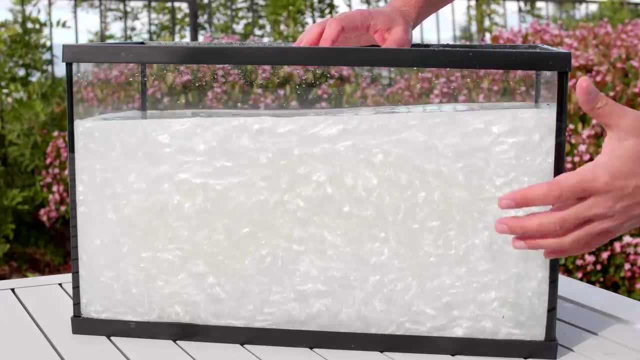 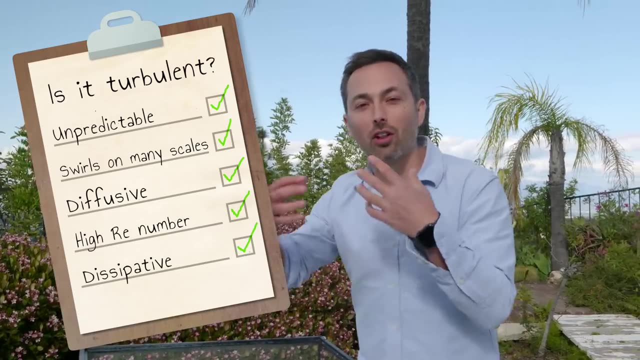 look at this turbulent flow is that it gradually dies away, and that's because another characteristic of turbulence is that it's dissipative. that is, it takes in energy at the largest scales, at these big eddies, and then that energy gets transferred down to smaller and smaller eddies. 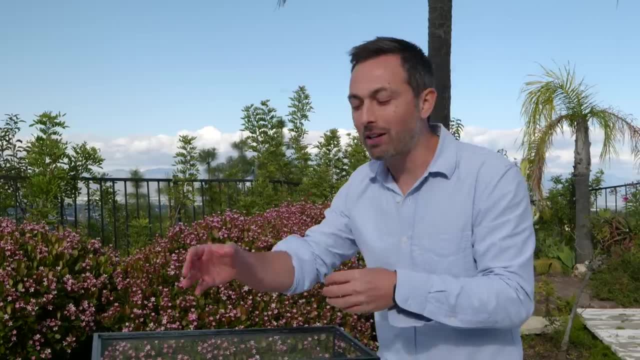 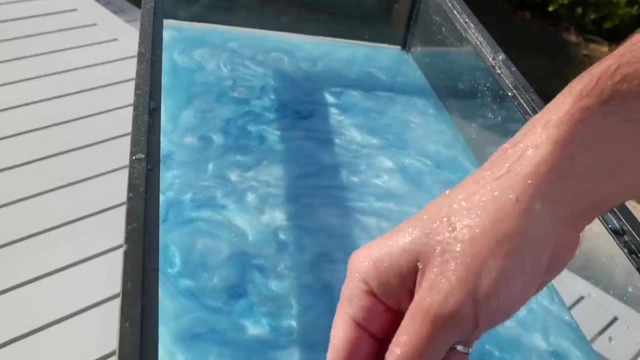 until on the smallest scales, that energy gets dissipated to the fluid as heat, and so, in order to create turbulence, you need a constant source of energy, something to keep generating those large eddies, which is why we often think about turbulence around objects that move through a fluid. 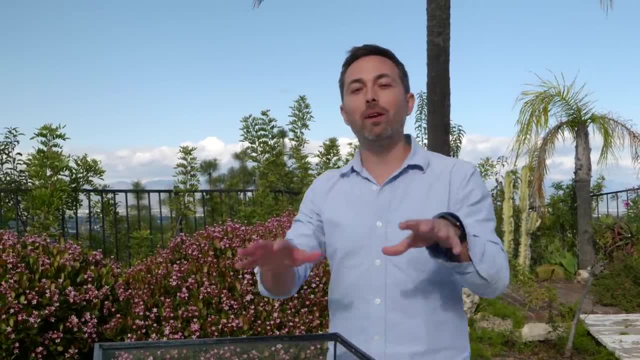 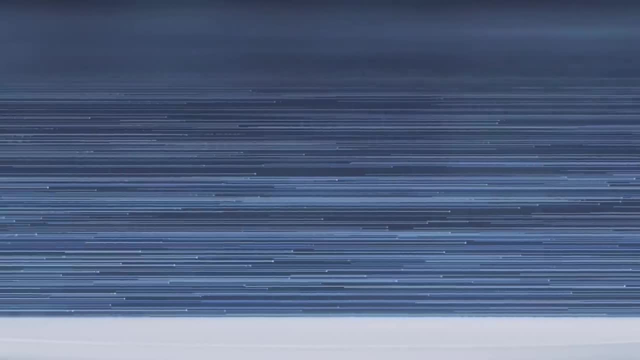 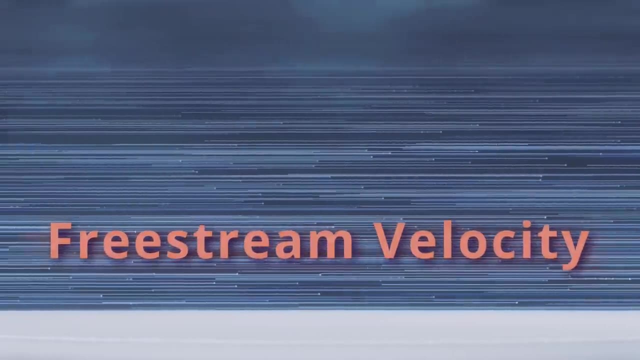 things like planes, cars or boats. so i want to think about the interface between an object and the fluid. so picture fluid flowing over a flat surface, far away from the surface. the fluid isn't affected. it keeps moving with what we'll call its free stream velocity, but right at the surface due to 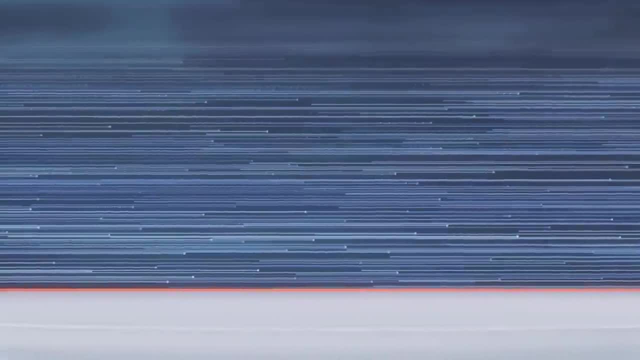 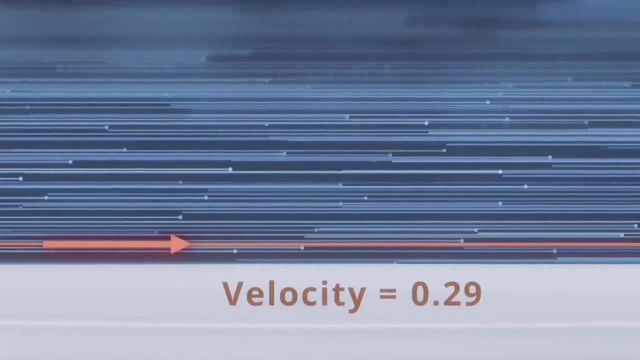 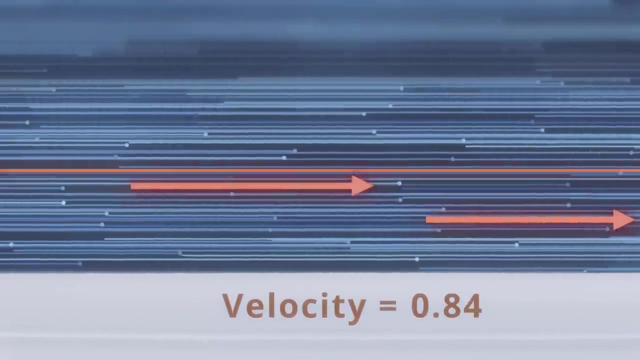 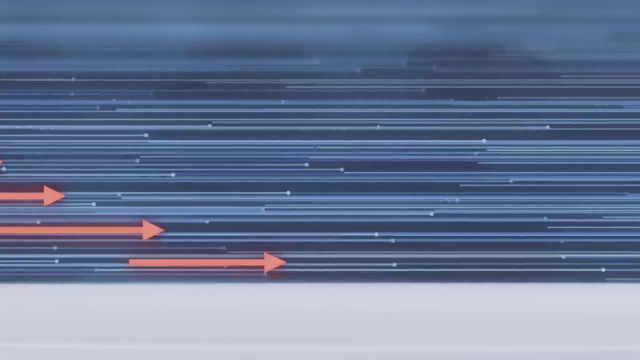 friction and adhesion, the molecules of the fluid are effectively stuck to the surface. their velocity is zero. the fluid next to it can flow only slowly due to friction with this stationary layer. with increasing distance from the surface, the fluid's velocity increases from zero until it reaches the free stream velocity, and this region of velocity adjustment is known as a. 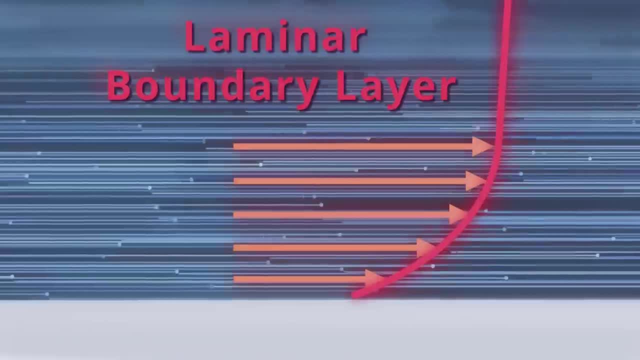 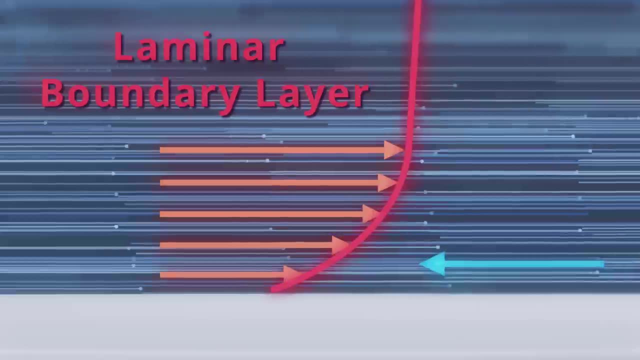 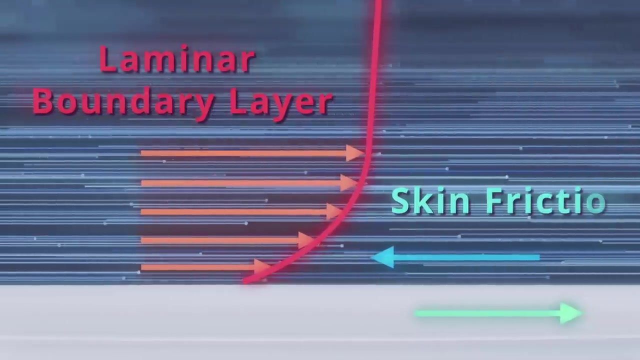 boundary layer. in this case, it's a laminar boundary layer. to form this boundary layer, the surface is applying a force to the fluid. that means the fluid is applying an equal and opposite force on the surface, and this is known as skin friction. now, if the fluid velocity is particularly fast or if the surface is long, 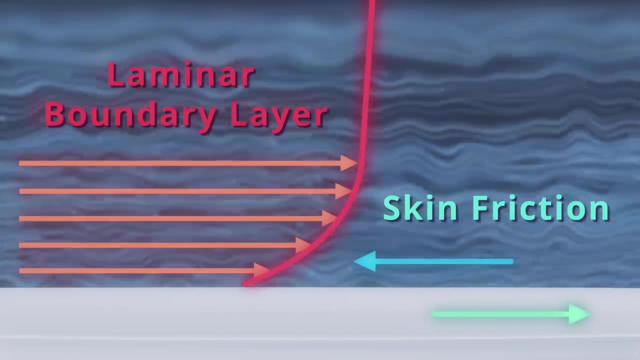 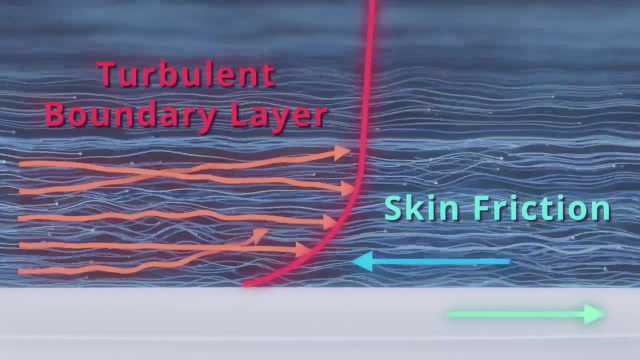 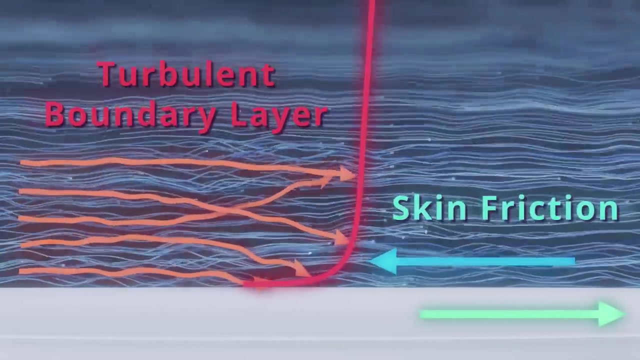 the boundary layer will grow and eventually transition to turbulence. in a turbulent boundary layer, the fluid swirls and mixes, bringing faster flowing fluid closer to the surface, and this increases the skin friction. so turbulent boundary layers result in significantly more drag than laminar ones and the boundary layers around planes and 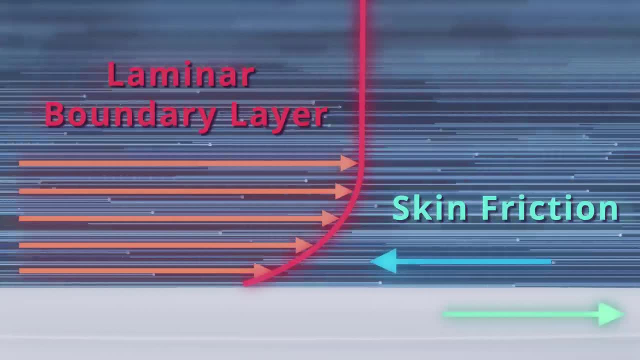 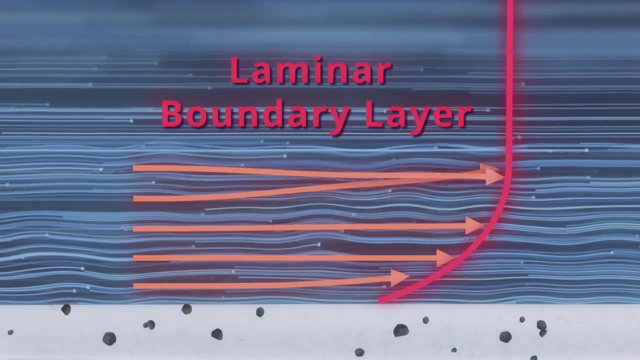 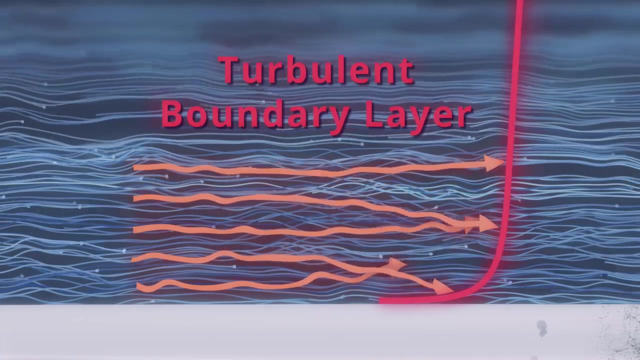 large ships are mostly turbulent and skin friction accounts for the majority of the drag they experience. to make matters worse, laminar boundary layers can be tripped into becoming turbulent by small obstacles or rough surfaces. in practice, this means clean, smooth surfaces can significantly reduce drag, saving on fuel costs if your car is really dirty. 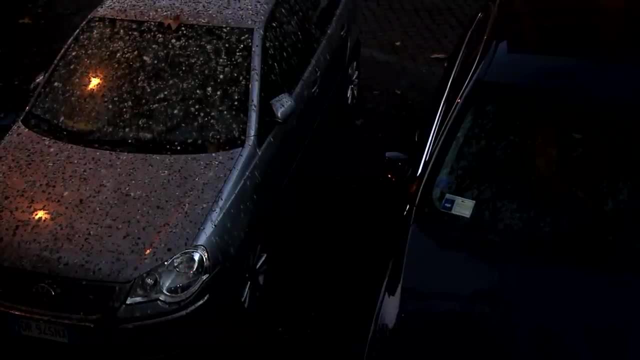 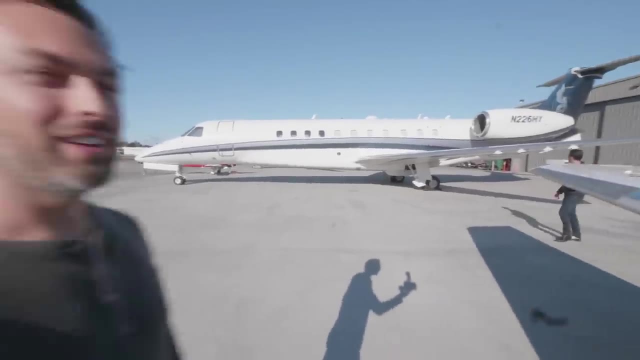 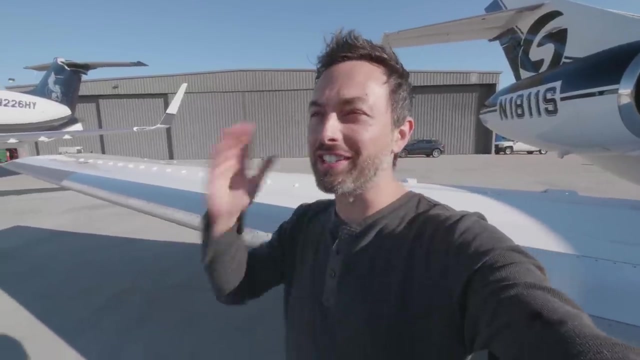 it likely gets worse gas mileage than if it were clean. this is what the mythbusters found when they tested it. it also explains why planes are frequently washed. so when you think about airplanes, i imagine that they will be built as smooth as possible. i think of the scene in the aviator where leo says he wants all of the rivets shaved down flush. 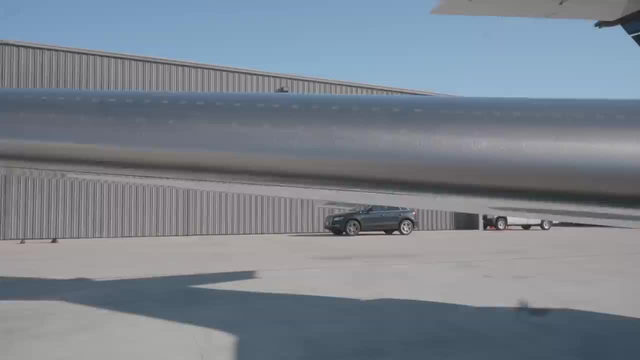 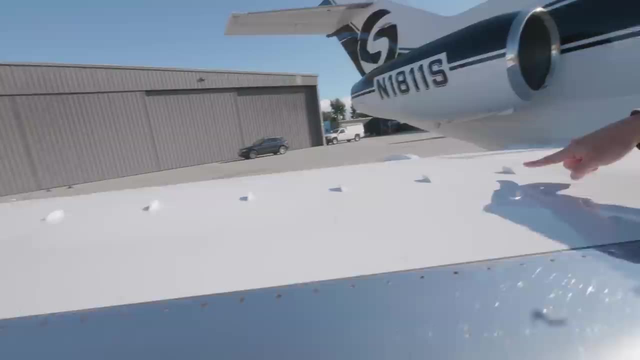 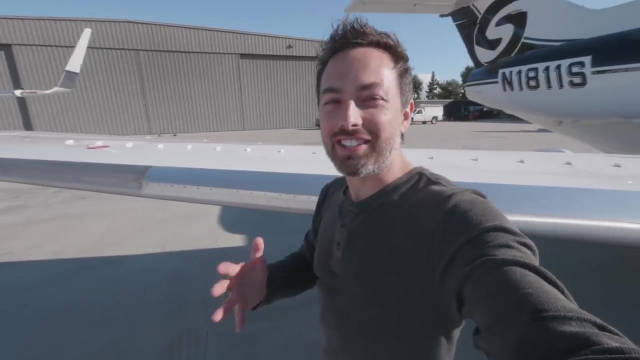 and you can see that with this plane, all of these screws are are set in to the wing and really to make the smoothest service possible. but then you look over here and there are these ridges that stick up out of the plane which seem to make no sense. i mean, why would you add roughness to the surface of the wing? the answer: 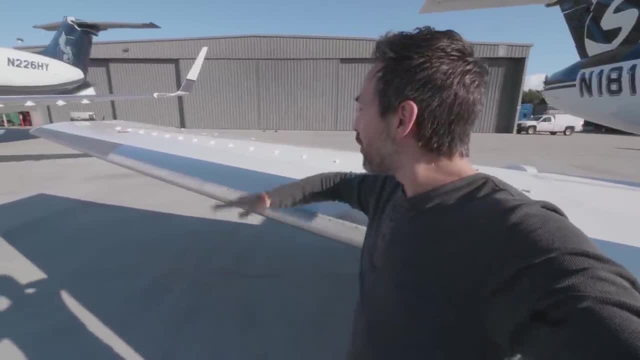 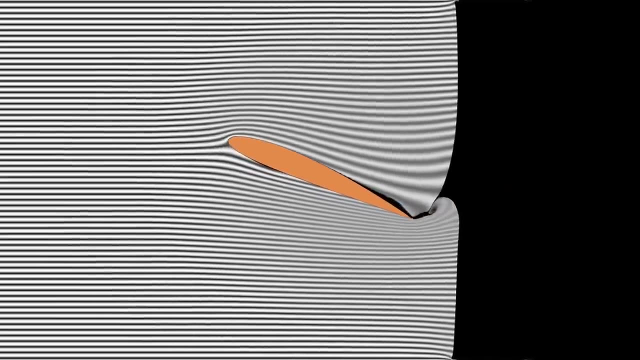 is actually to induce turbulence in the flow of air over the wing. when cruising in level flight, air smoothly follows the current and the wind follows the current and the wind follows the current curve of the wing. but at low speeds or higher angles of attack, the airflow can separate you. 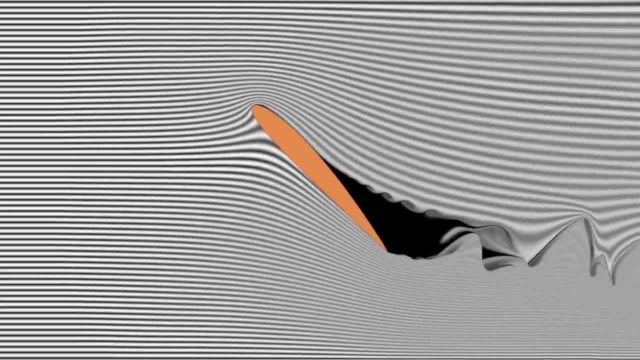 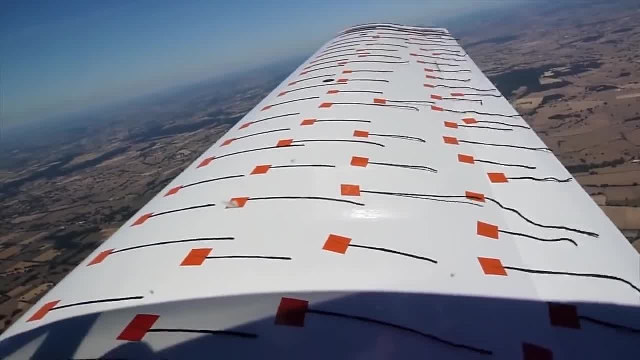 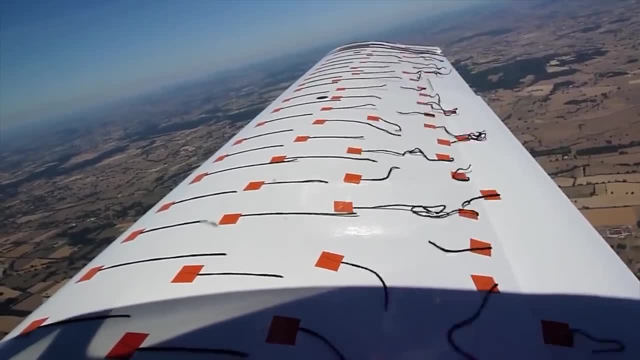 can think of it as not having enough energy to follow the curve of the wing. this leads to a condition known as stall, which dramatically decreases lift. here you can see the airflow via strings taped onto the wing and as the plane slows, the flow separates and the strings go wild. 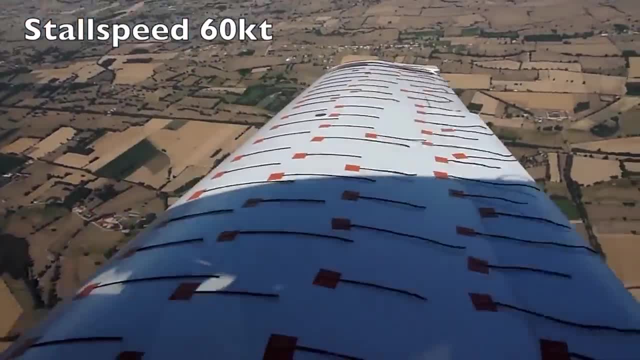 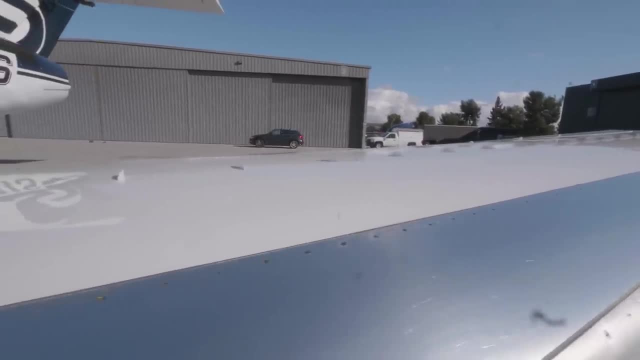 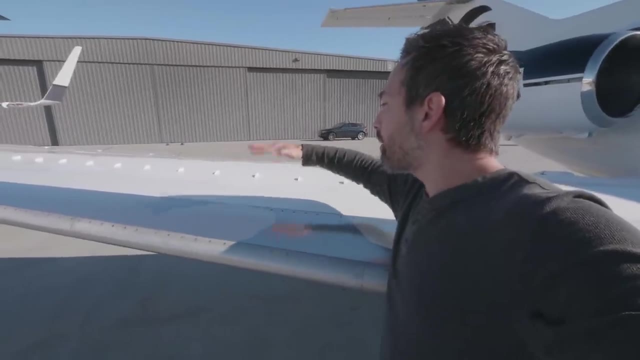 this plane has stalled. the way to delay flow separation and stall is by adding small fins on the wing, called vortex generators. what these vortex generators do is they actually cause turbulence which mixes the faster flowing higher up air down closer to the surface. so you're energizing that fluid flow as it passes over the wing. 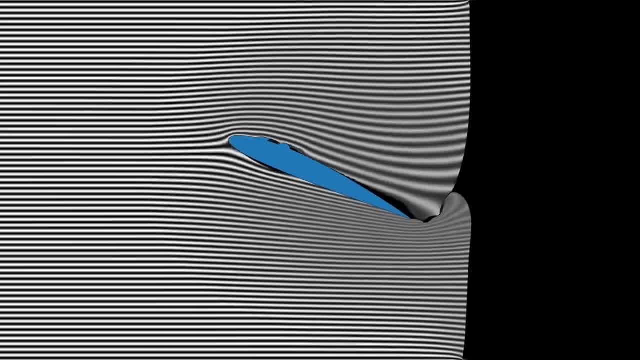 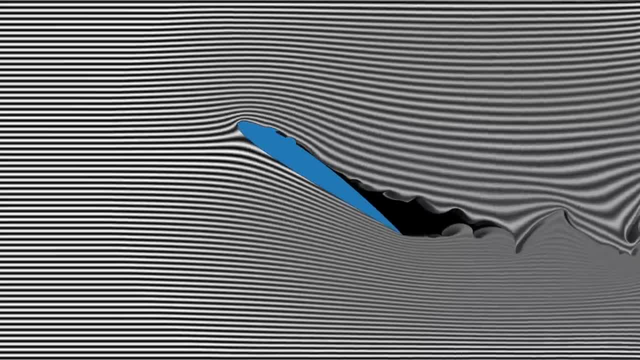 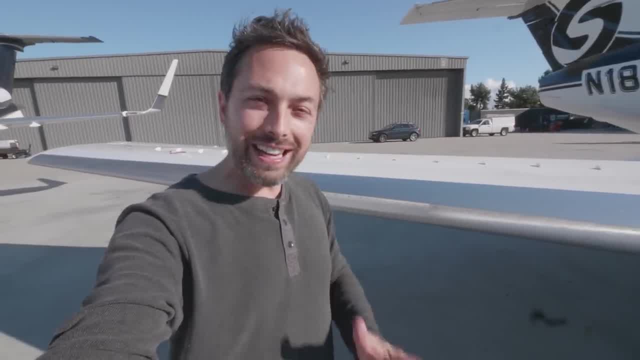 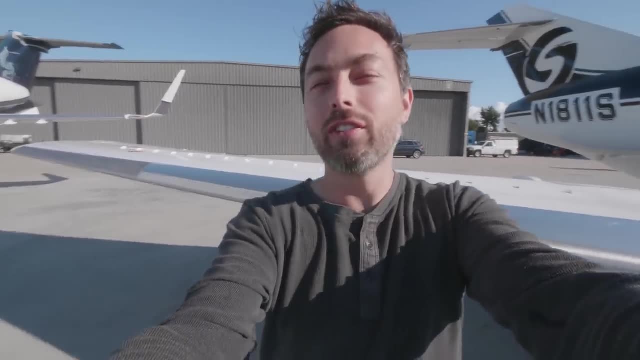 and because that flow has greater energy, it is able to follow the surface of the wing for longer. that means the airflow remains attached and if you have attached airflow over the wing then you can maintain lift. so in the case of airplanes, you actually need turbulence and you induce more turbulence on the wing- in order to fly efficiently and effectively and be 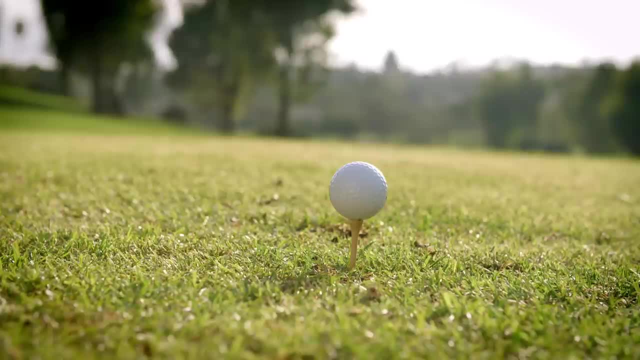 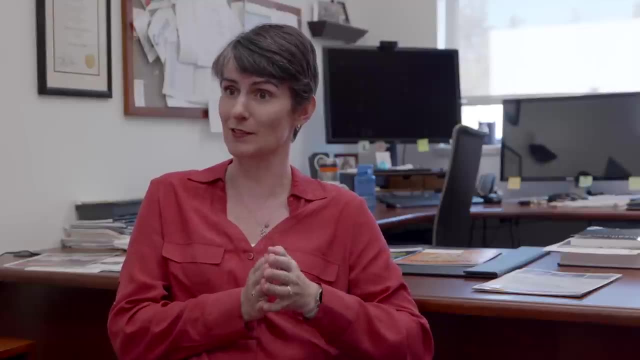 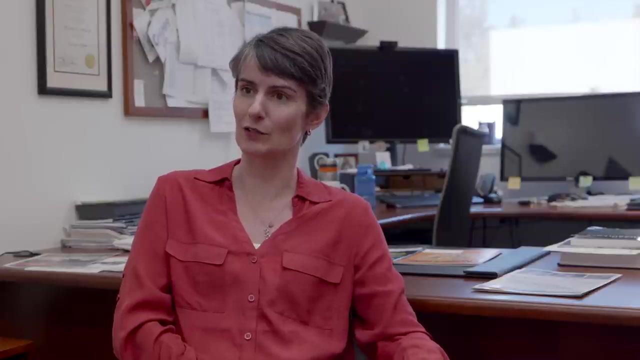 able to climb at higher angles of attack. a similar principle is at work with golf balls. the scots found out about turbulence the hard way because they started playing with a very smooth golf ball and it wouldn't fly as far as it would once it got sort of dinged and nicked and dirty. you can see why by observing the airflow in. 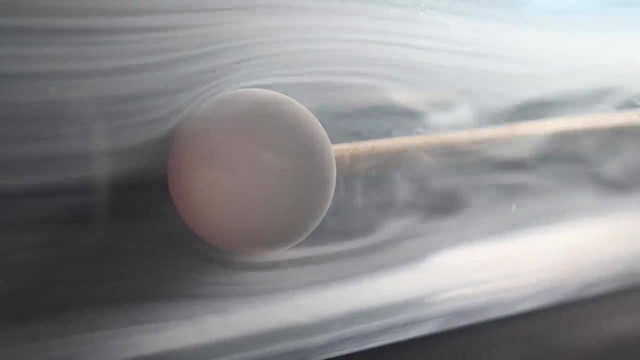 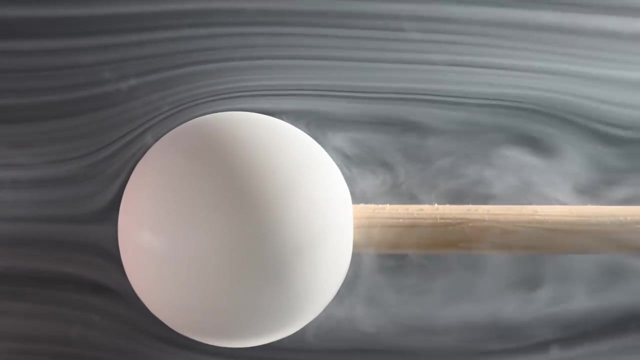 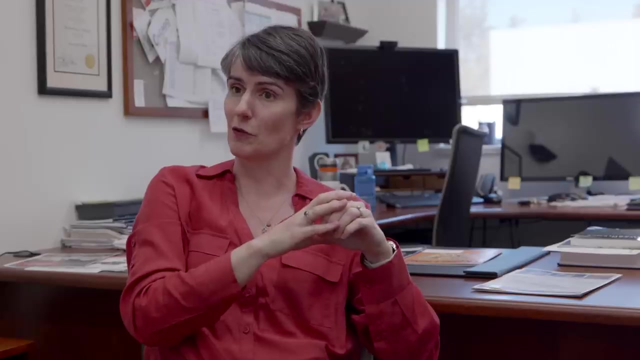 a wind tunnel with a smooth ball, the air forms a laminar boundary layer over its surface. this leads to low skin friction, which is a good thing, but it also means the airflow separates easily, leaving a large wake of low pressure, turbulent air behind the ball, and that leads to a different form of 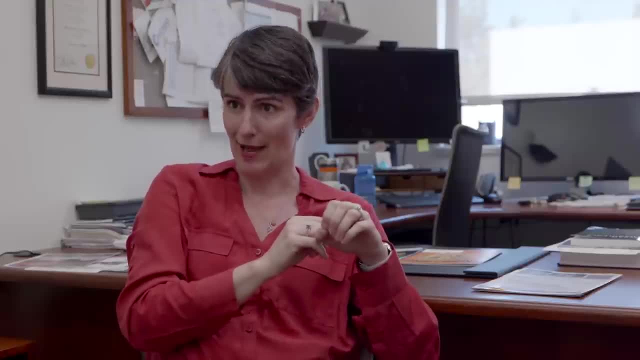 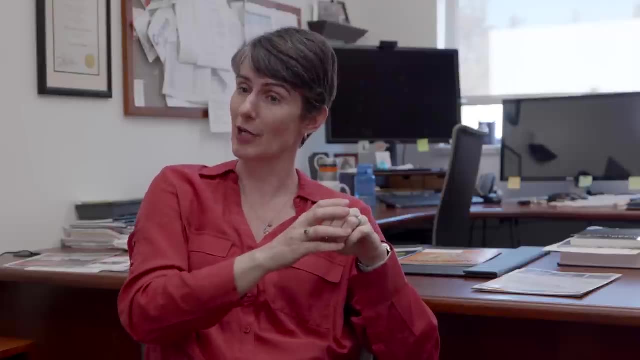 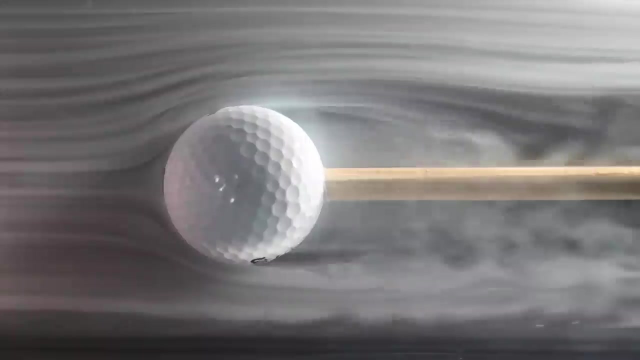 drag. is that a pressure difference? drag, that's right, that's a pressure drag. so the boundary layer itself has a skin friction drag and then if it separates, there's a pressure drag. and if you force that boundary layer to become turbulent, so you have mud or roughness or nicks, 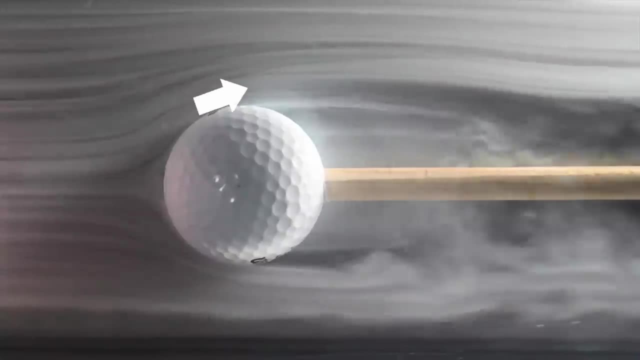 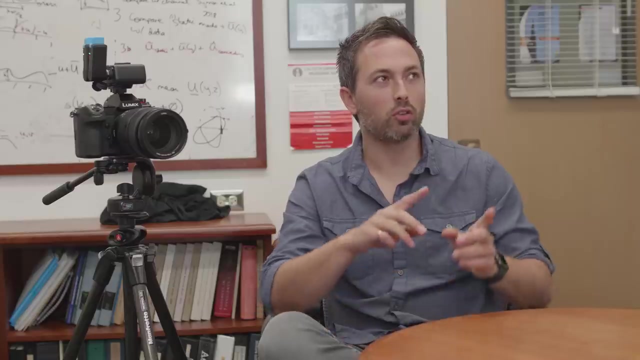 on the golf ball, then a turbulent boundary layer can actually get further around the golf ball before it separates, and so it reduces that wake and reduces that pressure drag. so by reducing the pressure drag it's more than you're increasing the skin drag. that's right. golf ball travels further. golfers started carving grooves into their golf balls before the aerodynamics of this was fully understood, and since then dimples have found to work the best for creating a turbulent boundary layer. dimples are very shallow compared to the diameter of the golf ball, but they have a pretty 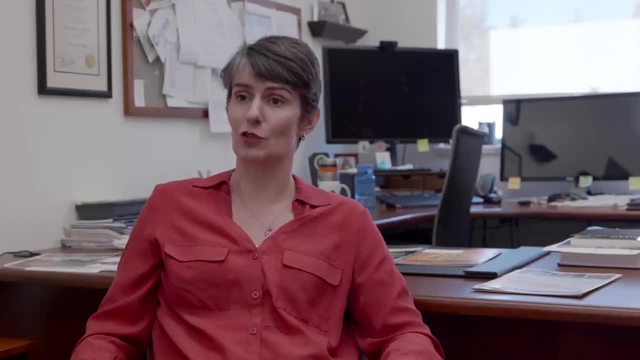 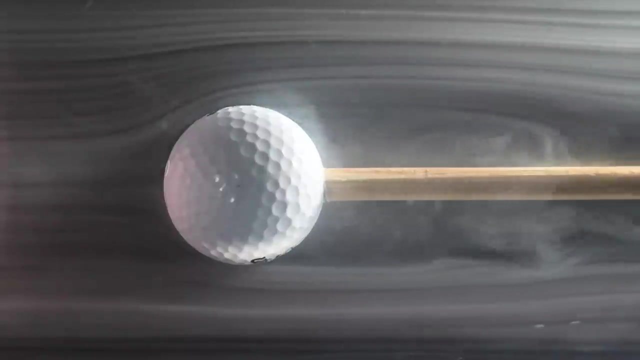 massive effect. what sort of effect are we talking? looking at the drag, what we call a drag coefficient, you see a really big drop, almost a factor of two, when the boundary layer becomes turbulent. so having a turbulent boundary layer reduces the size of the turbulent wake, but turbulent wakes themselves are 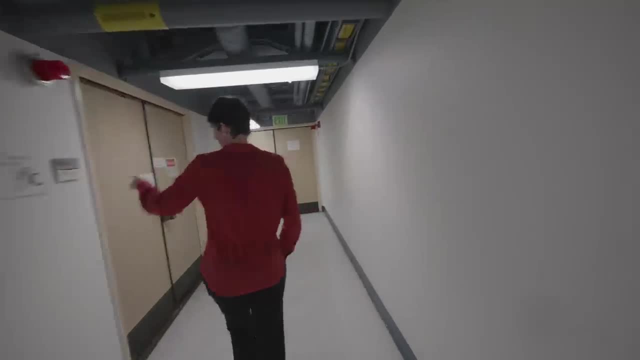 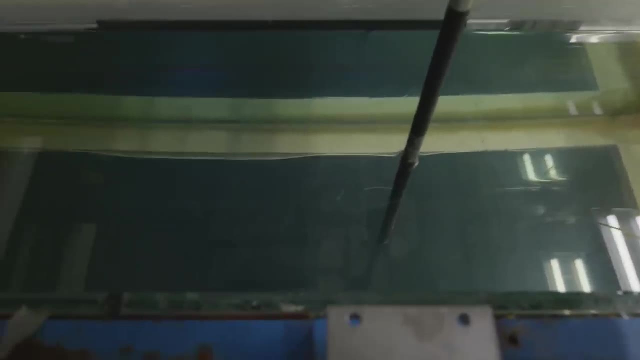 interesting and scientists are looking for ways to harness the energy they contain. there's a lot of water here. i came to caltech to see this experiment where the water flows around a cylinder and transitions to turbulence in its wake. the flow is visualized here using a fluorescent dye. you can 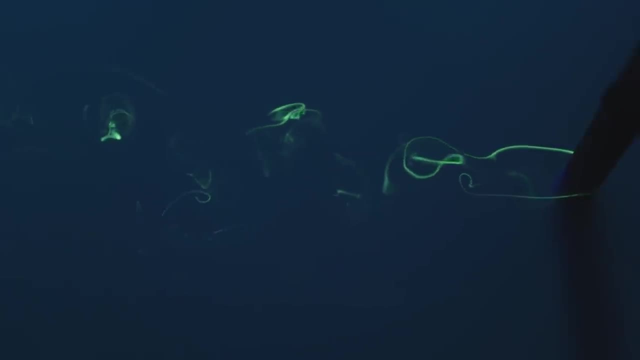 see how, under the right conditions, vortices are shed by one side of the cylinder and then the other, alternating back and forth in a regular pattern. this is known as periodic vortex shedding, and the pattern it creates downstream is called a von kármán vortex street. these patterns appear all over the place most. 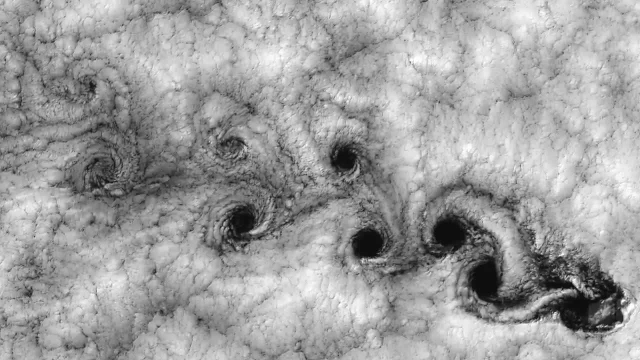 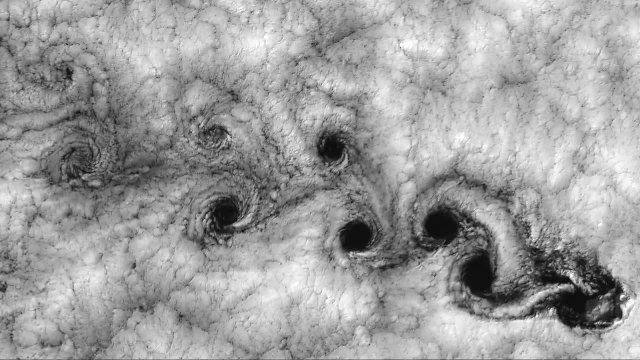 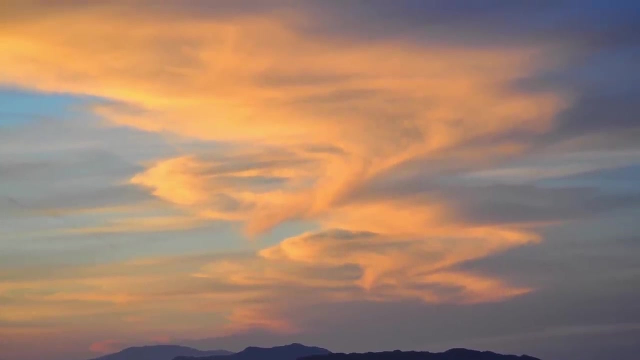 spectacularly in images taken from space. at this scale, an island acts as the obstacle that creates the periodic vortex shedding, and the vortex street is made visible by patterns in the clouds. these patterns can even be seen from ground level. obviously, this phenomenon is not strictly turbulent, because it follows a predictable. 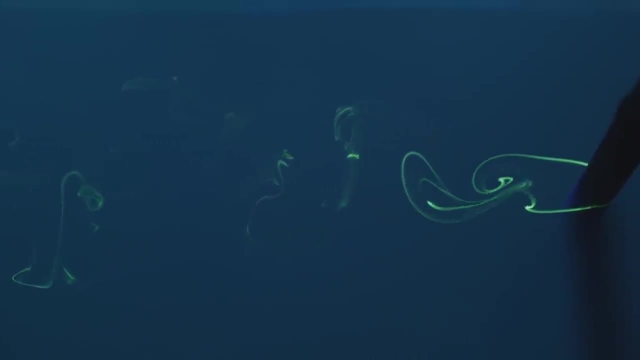 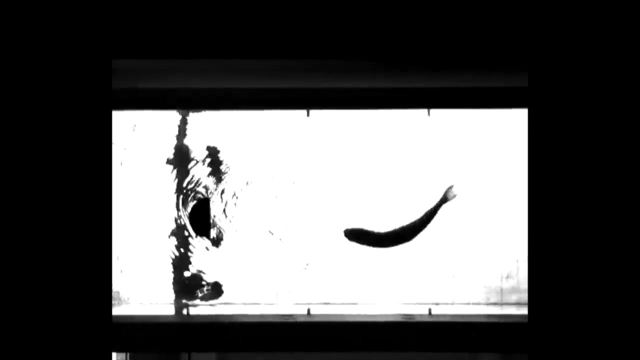 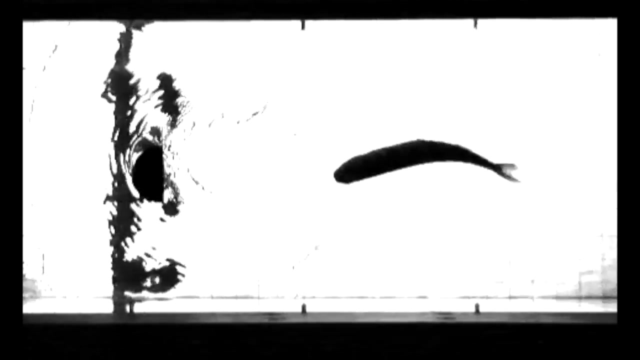 pattern, but it is part of the transition to turbulence and these scientists are looking for ways to harness the energy in these vortex structures. one experiment showed that if you put a dead fish in the wake of an object, it will actually swim upstream. this suggests fish can take advantage of turbulent water to swim more efficiently. it's just one way. 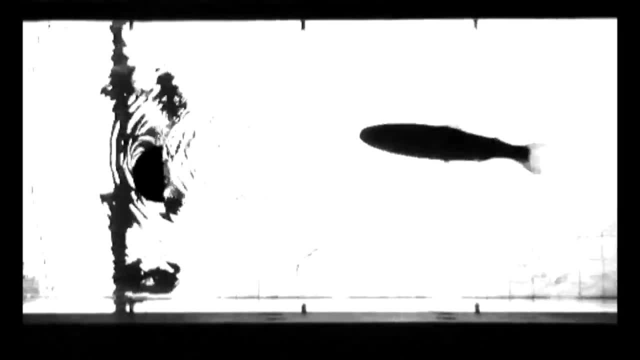 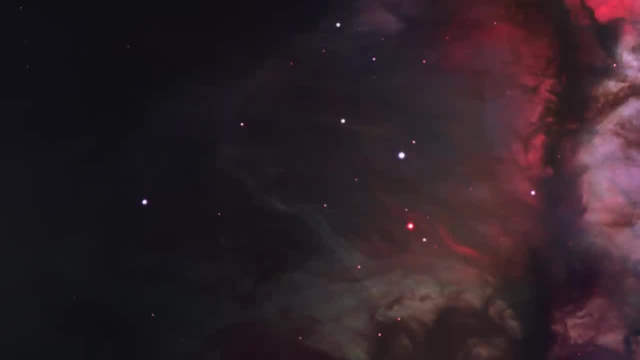 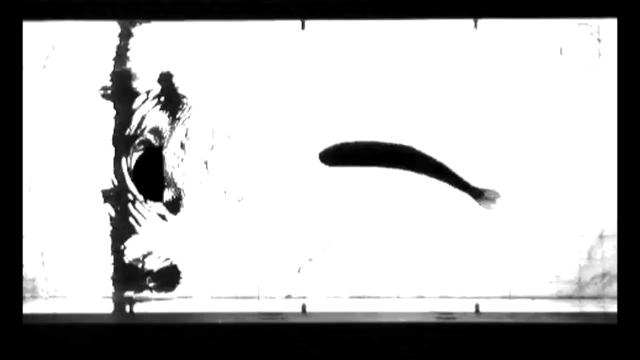 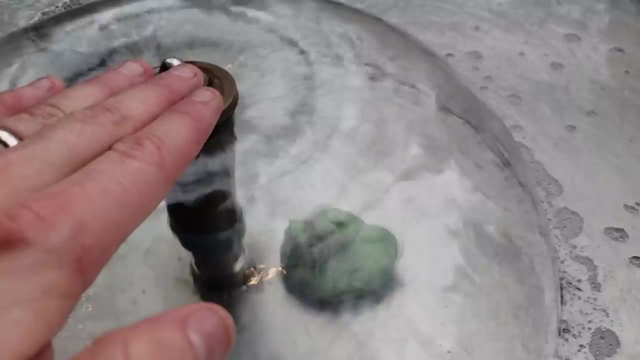 animals have adapted to live in a turbulent world. so, to sum up, turbulence is everywhere. it's inside you, around you, from the smallest scales up to the largest structures in the universe, and it's useful for flying airplanes, forming raindrops, making golf balls fly further and helping fish, dead or alive, swim upstream. in contrast, laminar flow is small, superficial. it's. 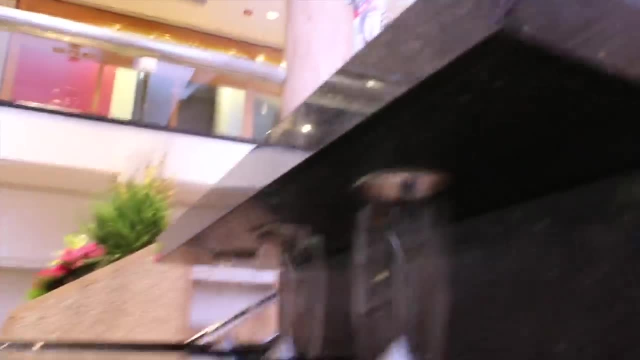 a toy. that's why its most notable use is in decorative fountains. and that's why it's most notable use is in decorative fountains, and that's why it's so important for us to be able to see what's in the water and what's not to be seen in the water, and what's not to be seen in the water and what's not to be seen in the water. 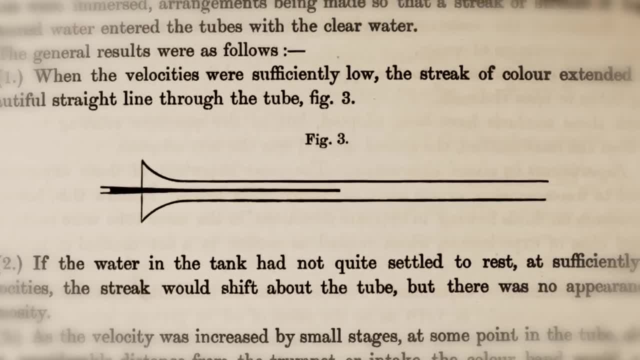 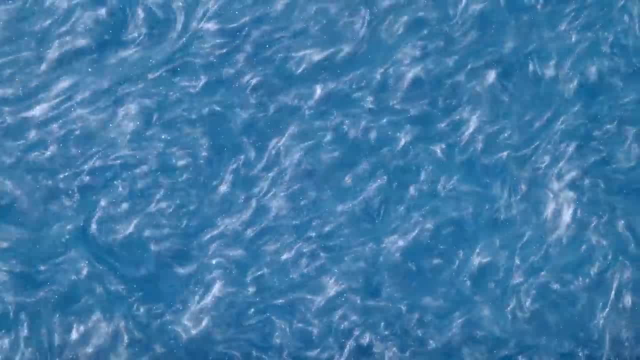 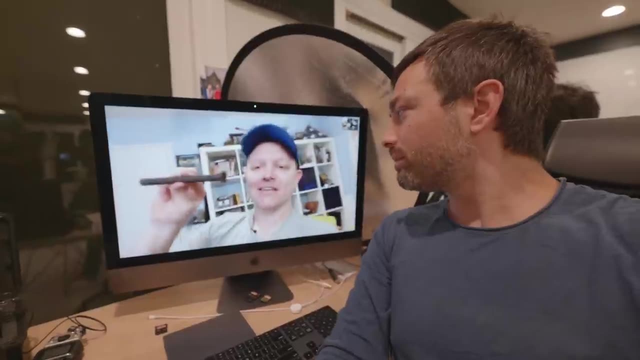 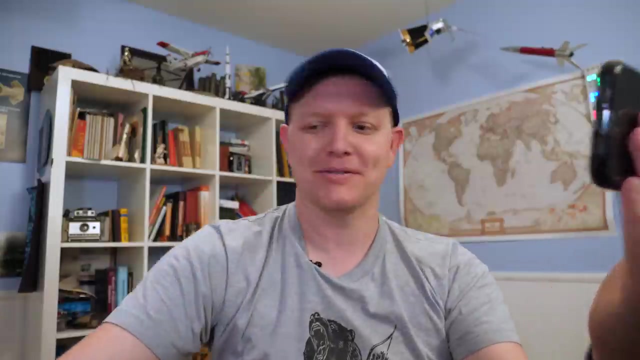 it appeals to your desire for order. but the world, like turbulence, is messy. that's why i personally prefer the richness, the unpredictability of turbulent flow. no, but. but turbulent flow has its places too. i'm actually like studying turbulent flow for, like my, my schooling, like i'm studying turbulent flow in rocket nozzles. 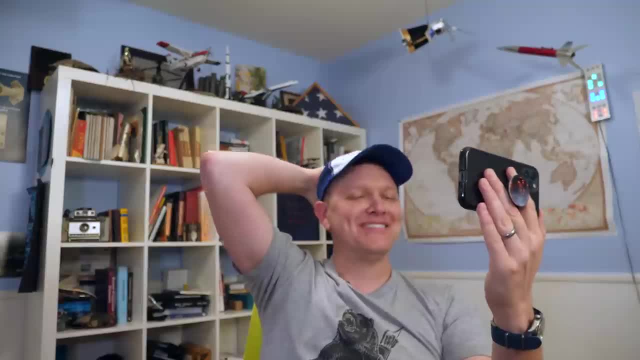 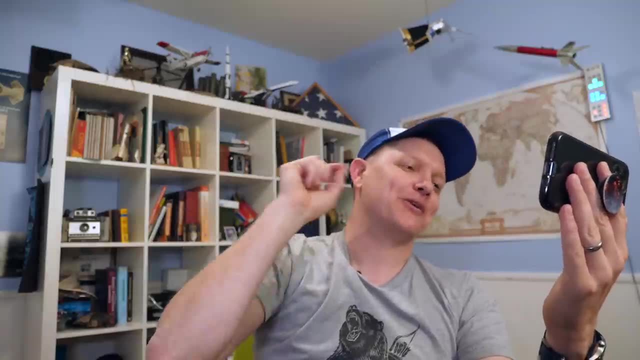 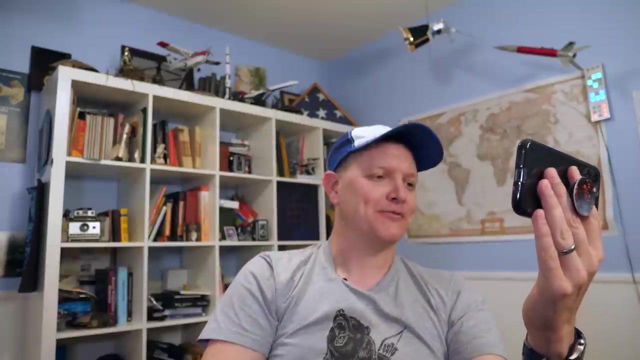 that's a thing you're cheating on. laminar flow is what you're doing. um, no, yes, yes, maybe i don't know, uh, but you will not get me to say turbulent flow is not awesome and not beautiful. you will not get me to say that. so i will concede, and i agree with you: turbulent flow. 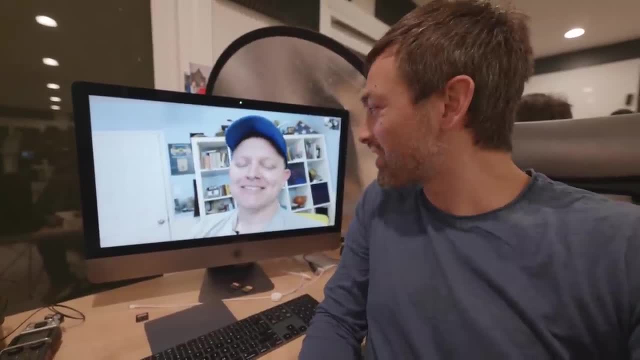 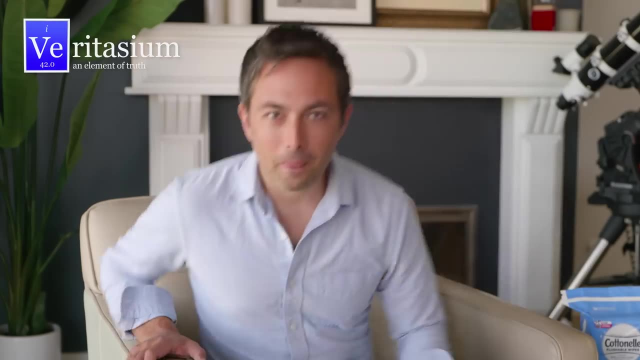 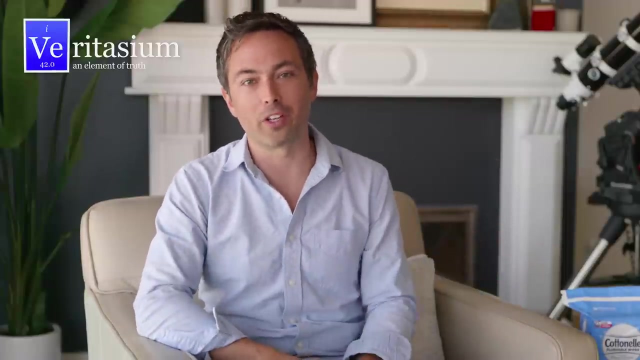 is awesome, i will agree. all right, all right. well, it's just not as awesome as laminar flow. let's be honest. hey, i just wanted to let you know that this video was filmed before the covid outbreak and before the shelter-in-place guidance was put into effect. now, this portion of the video was 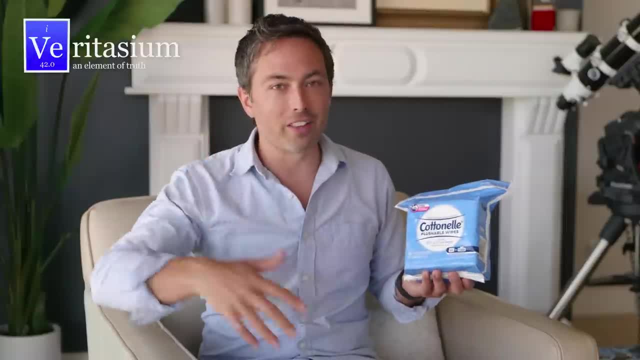 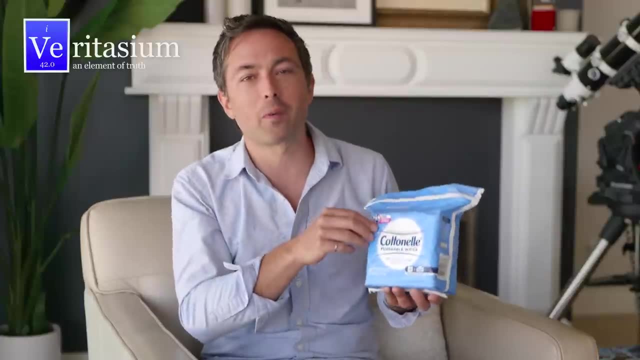 sponsored by cottonel flushable wipes and since the outbreak they have been working around the clock to get their products back on shelves and back. when i filmed this video, i actually did a little experiment with these wipes to find out how flushable they really are, so let's check that out. 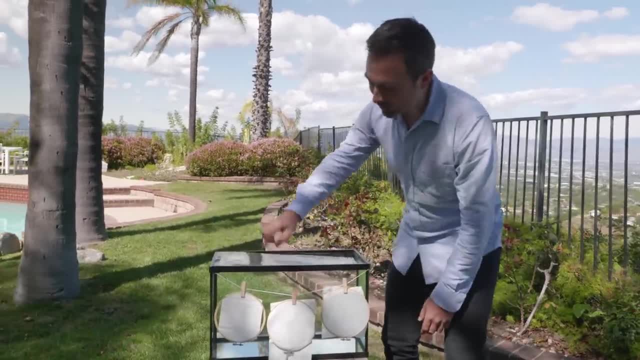 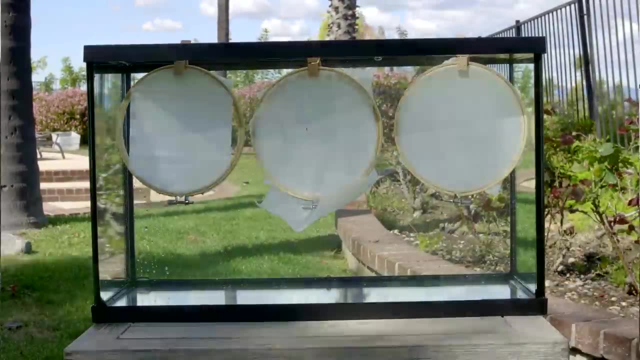 so here i have a baby wipe, a paper towel and a cottonel flushable wipe and i'm gonna submerge all three of these in the fish tank for 30 minutes and then the Danger to look, recording and then test how strong they are. Flushable wipes actually became really important to me. 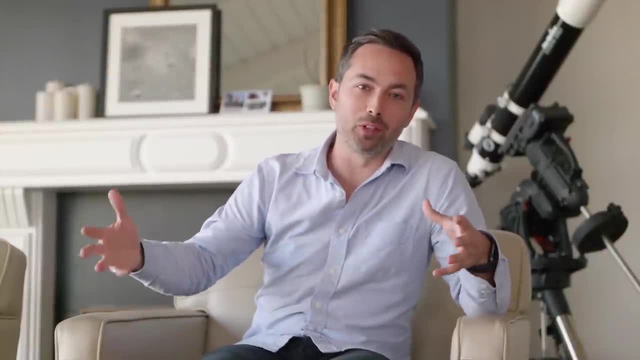 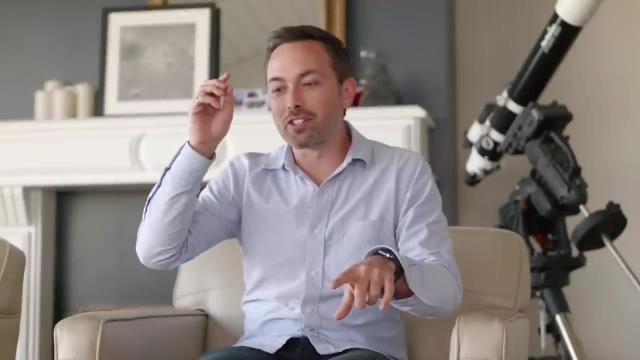 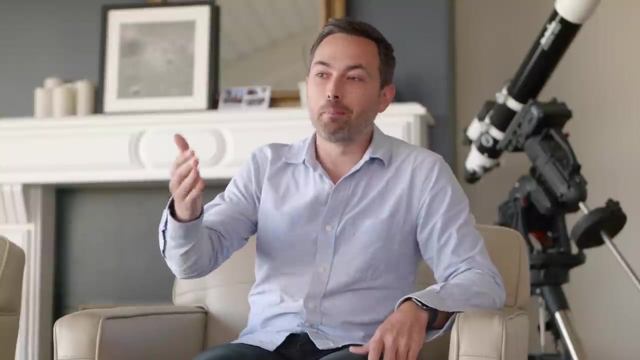 a couple of years ago when the main sewer for my building backed up into my condo and flooded the entire downstairs And the reason was my neighbor was flushing baby wipes down the toilet and that blocked up the whole system. So it was pretty awful, But in fact this is a thing people do a lot. 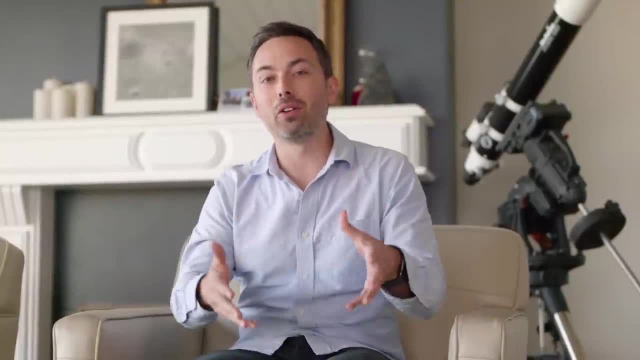 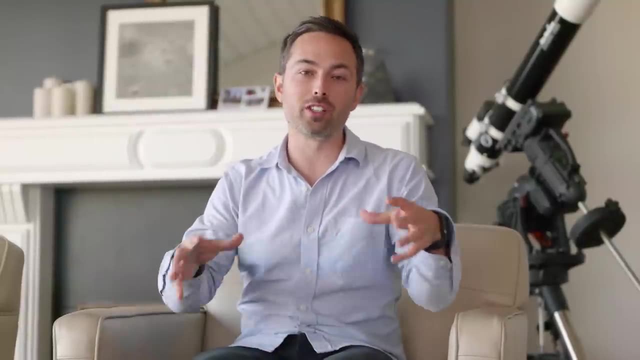 There was this study from 2016 that found in the US, 60 million baby wipes are purchased every year and 7 million of them end up being flushed down the toilet. In fact, when they looked in the New York City sewer system, they found that 38% of the stuff you find in there is actually these baby wipes. Meanwhile, 14 million flushable wipes are purchased every year and flushed down toilets, but they make up only 2% of what you find in the sewer system.